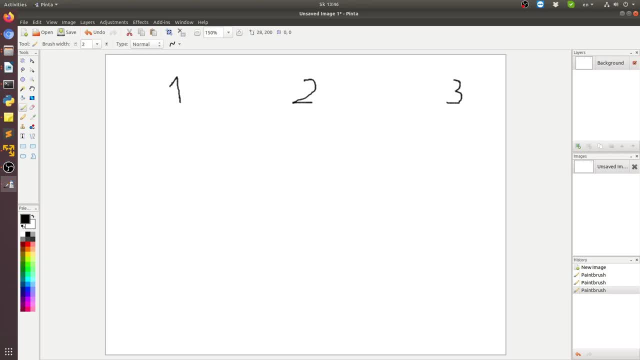 highest current payout average with probability 20%, for example. So it's much easier to understand with concrete example. suppose, after our first vocals we played machine one four times and we won one dollar two times. so we can write it out: we played, for example, uh, two times and we won one. 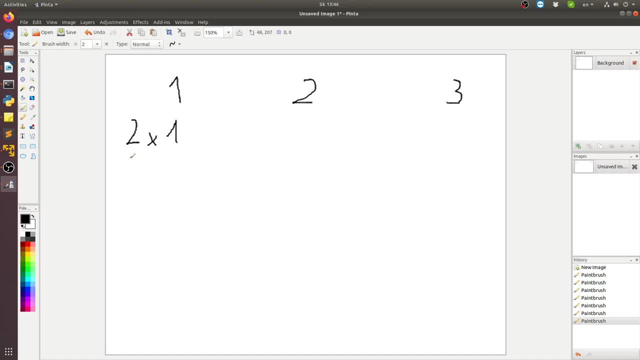 dollar and we played more two times and we won zero or we lost both times. so we'll drop zero here. the average win rate for this machine is 0.5. that's right, and and suppose we played machine two, five times and one, one dollar three times and zero. 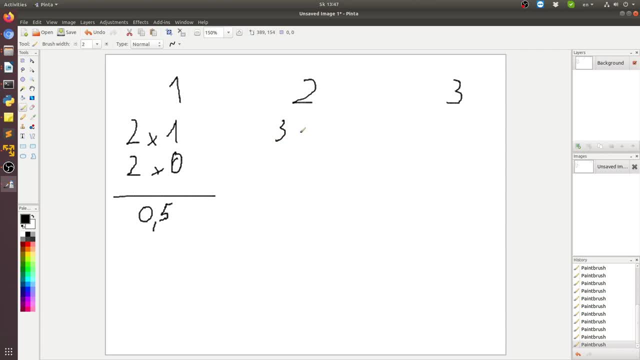 dollar two times, so i can write it something like three, three dollars and two times nothing. so for my drawing it's horrible, but it is how it is, and the average payout for this machine will be 0.6, 0.6, just like that, and suppose we played machine. 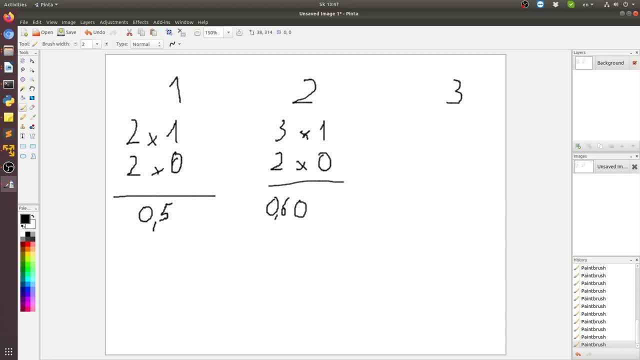 three, three times, and one. one dollar one time and zero dollars two times. so 1 x 1 will be and 2 x 0, and here i can write that average payout for this machine is 0.33. yep, that's right. now we have to select the machine to play. 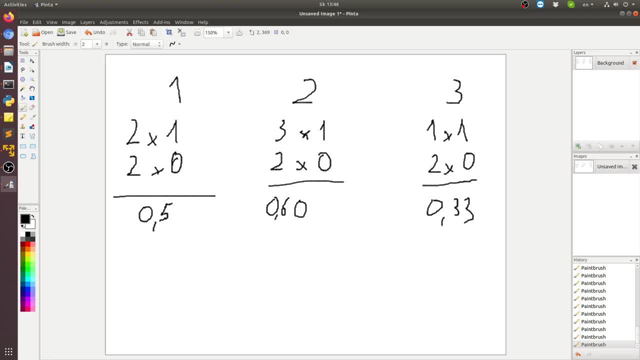 or we generate a random number, p between one zero and 100, for example. suppose we have set epsilon equal to, for example, 90, if random number is lower than 90, which will be 90 of the time, we select machine 2 because it has the highest current highest average payout but number higher than 90. 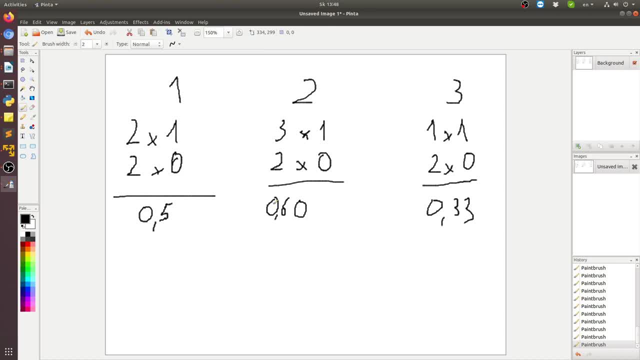 which it will be only 10 percent of the time. we select a random machine, so each machine has uh chance of being select one from three. so, shortly talking, we all the time play on this machine and and ten percent of times we choose randomly which machine we want to play. 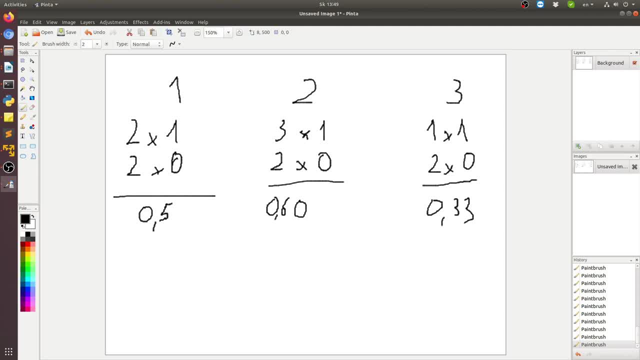 and notice that machine two might get picked anyway. because we select randomly from all machines. Over time the best machine will be played more and more often because it will pay out more often. In short, Epsilon Greedy means pick the current best option. I mean greedy most of the time. 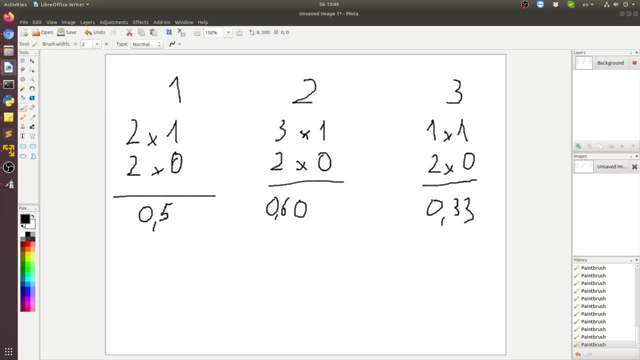 but pick a random option with a small probability. sometimes There are many other algorithms for the multi-armed bandit problem, but Epsilon Greedy is incredibly simple and often works as well as or even better than more sophisticated algorithms such as upper confidence-bound variations. 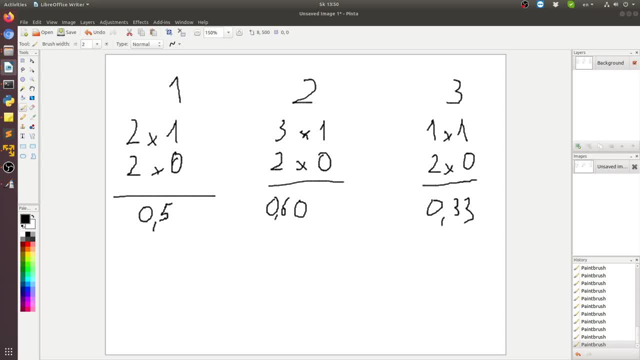 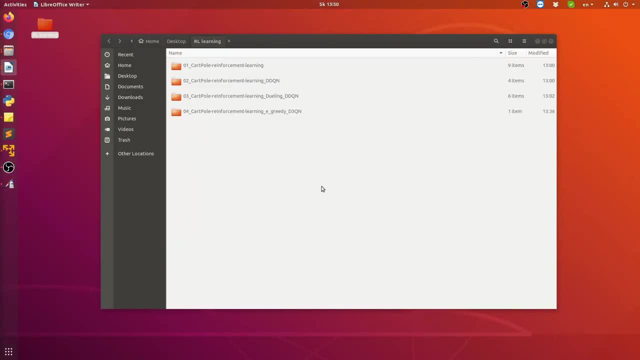 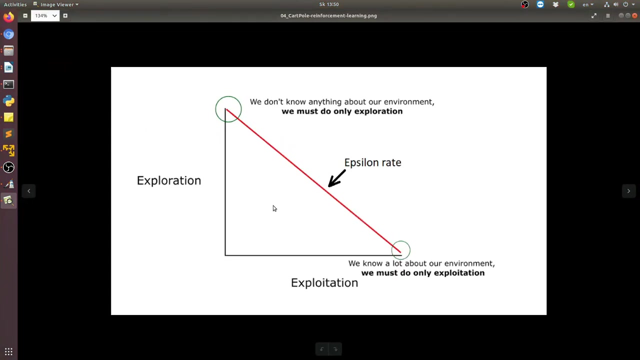 The idea is that in the beginning we'll use the Epsilon Greedy strategy and what we do, we specify an exploration rate, Epsilon, which we set to 1 in the beginning. so I can draw open you drawing and, yeah, I can maximize it, something like that. so we set one in the 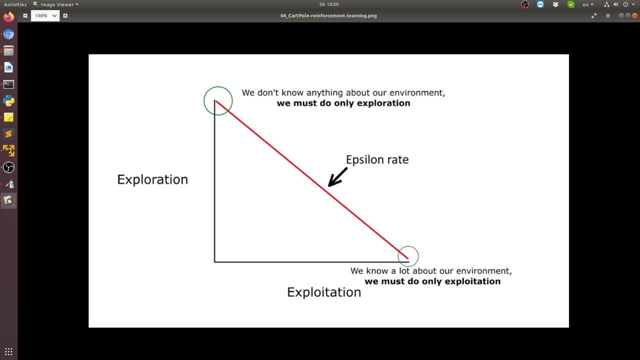 beginning. this is the rate of the steps that will do randomly in the beginning. this rate must be at its highest value because we don't know anything about the value in Q table. this means we need to do a lot of exploration by randomly choosing our actions so we generate a random number. if this number is more, 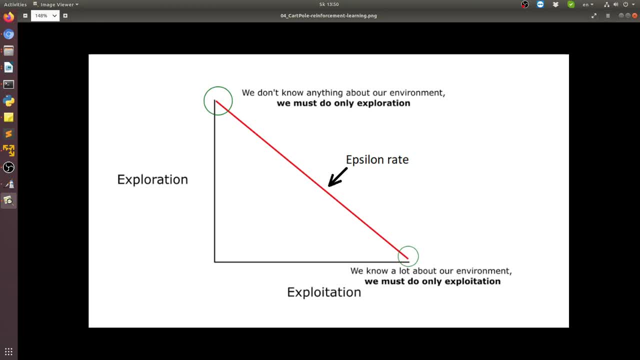 than epsilon, then we will do exploitation. this means we use that we already know to select the best action at each step, else we will do exploitation. so, as you can see, here is our exploration and exploitation and, for example, here is our epsilon, and it's depend what we'll do or what we random. 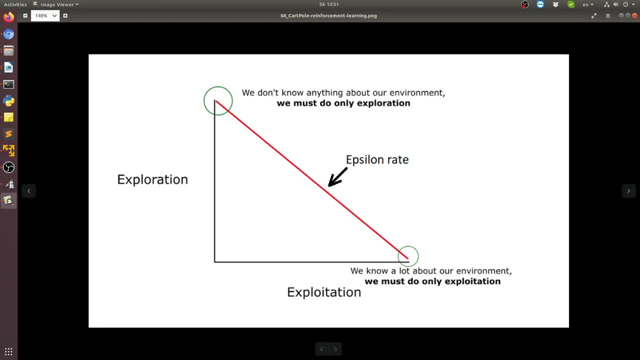 number we get. it's higher than, or higher than epsilon rate or lower than epsilon rate. the idea is that we must have a big epsilon at the beginning of the training of the Q function, then reduce it progressively as the agent becomes more confident at estimating Q values. so now 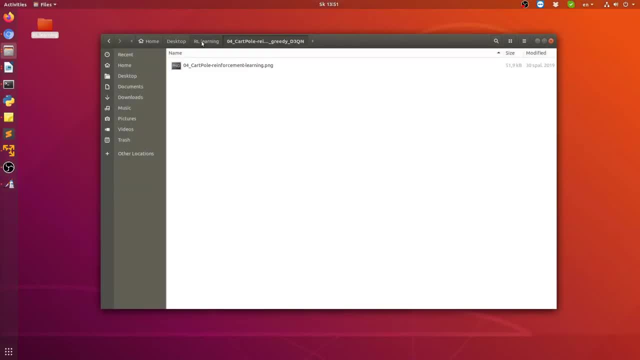 we can go to the code, as I showed us to you already. I'll copy my third tutorial code here. I can rename it to something like: right now it's: it will be these three and here will be epsilon, greedy strategy, something like that. oh shit, I need to remain or name it. 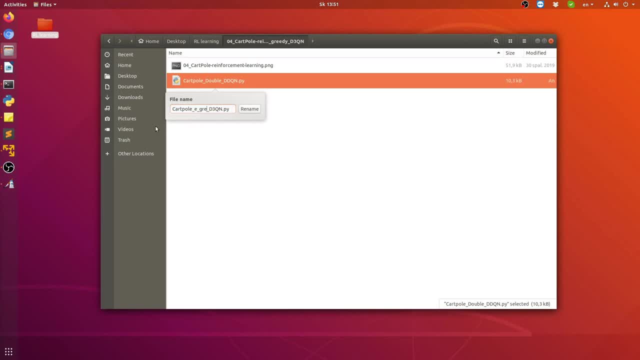 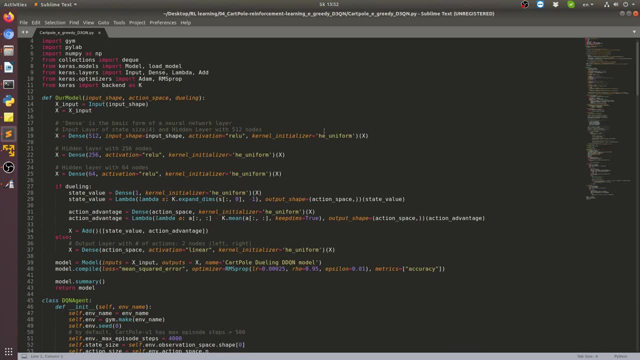 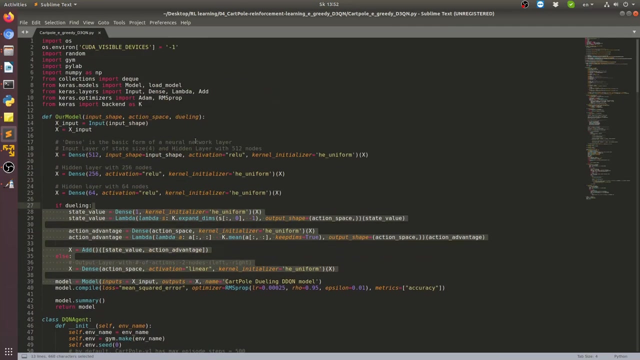 again double and epsilon, greedy rename, and let's open it with our sublime editor and so on, and we can begin somewhere. we'll keep almost all the settings in the code and we can start somewhere. we'll keep almost all the settings in the code and we can start somewhere. we'll keep almost all the. 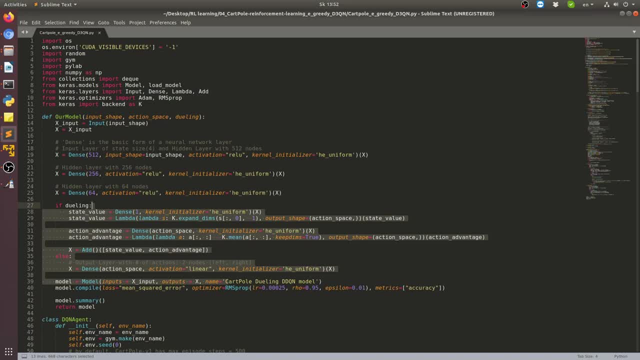 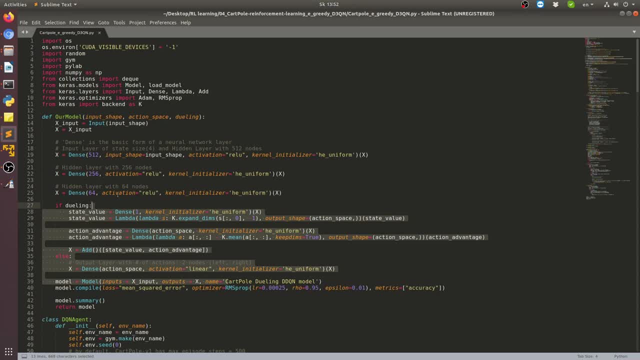 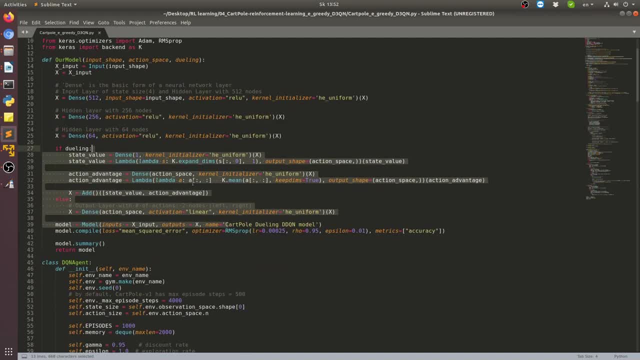 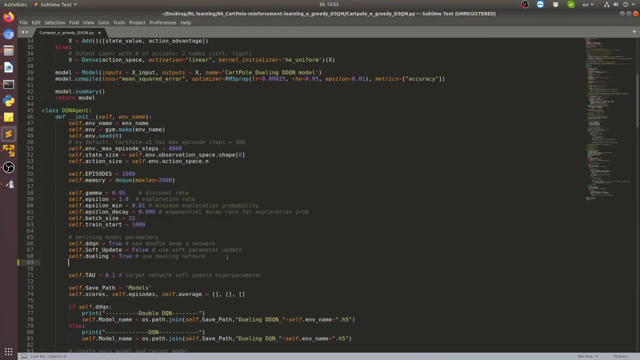 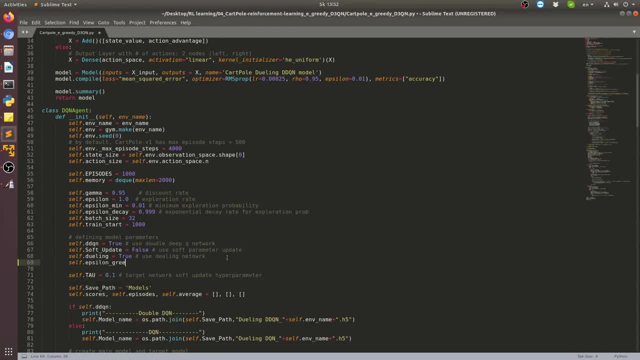 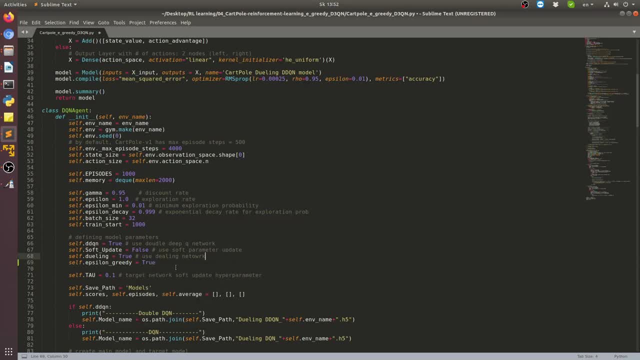 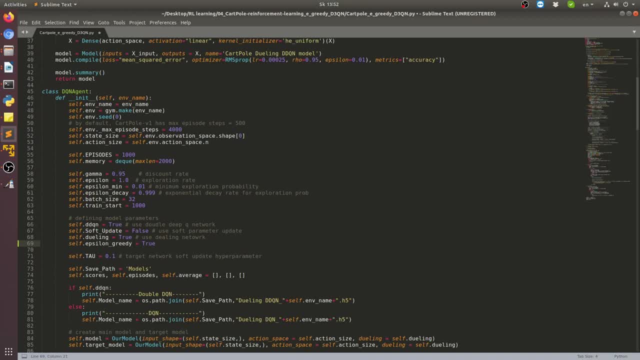 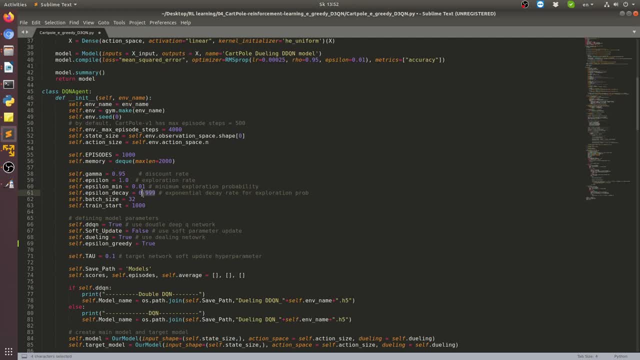 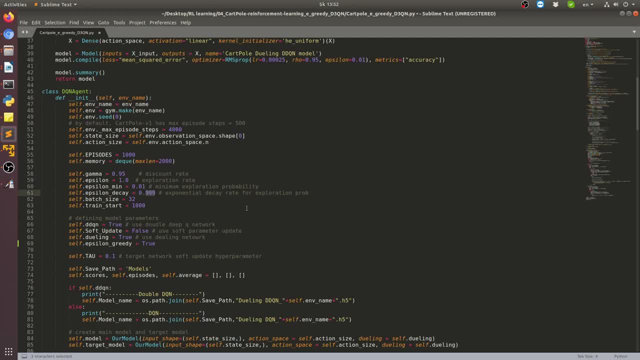 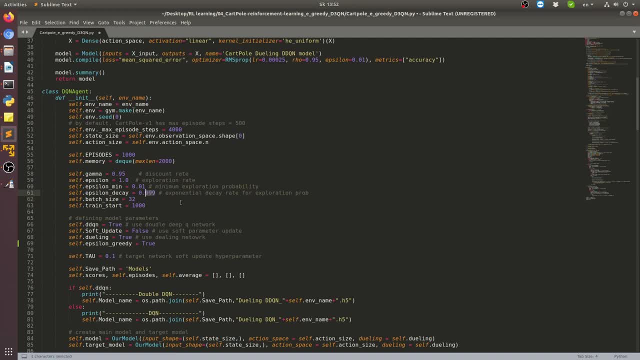 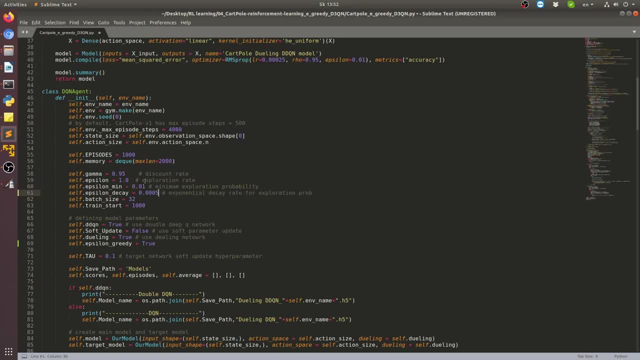 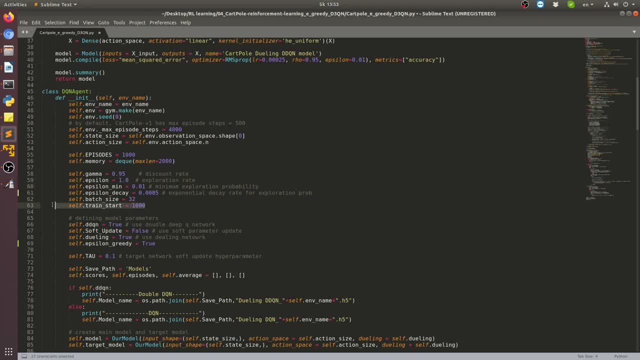 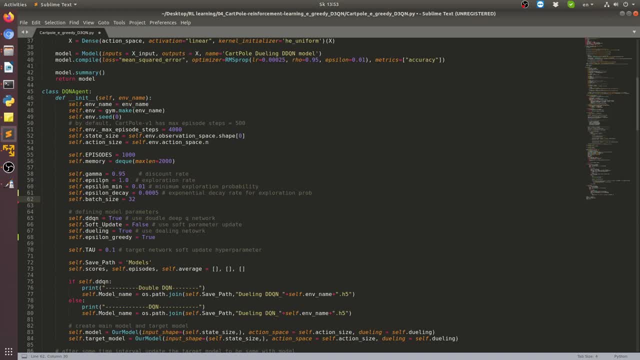 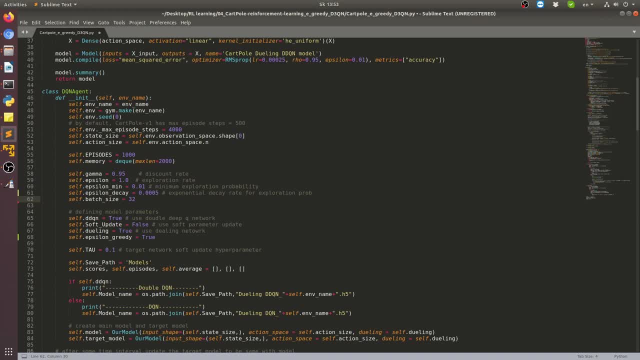 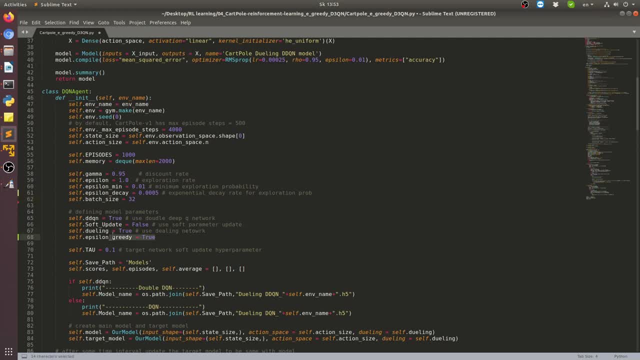 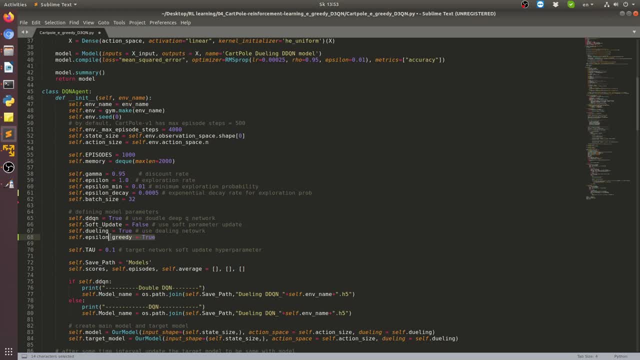 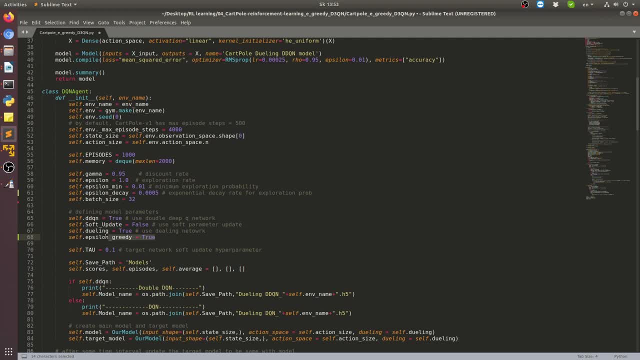 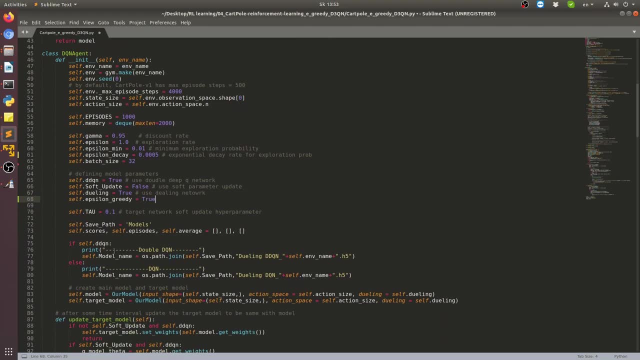 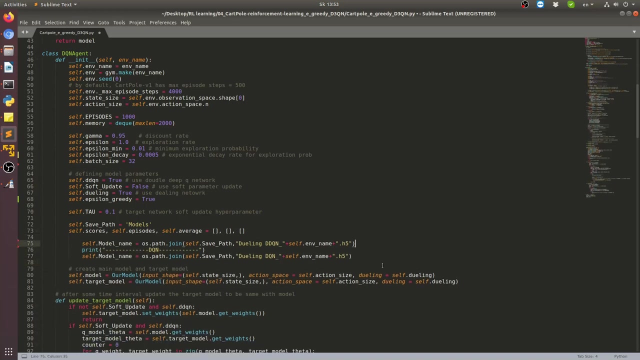 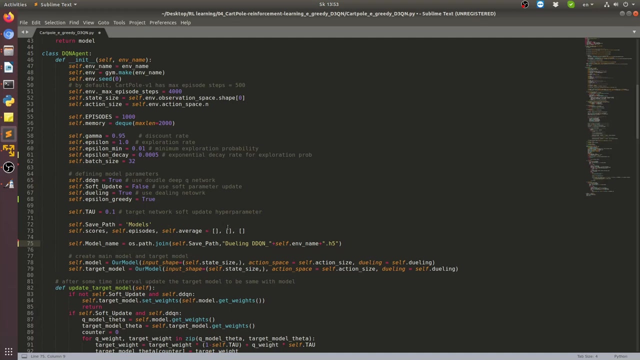 hyper parameters for epsilon and epsilon grid strategy will be quite the same. so what they change here, I I won't use this anymore. double or or not double, it doesn't matter. so I'll just remove this, this and this, and right now it will be simply a self model name, and here I'll use not dwelling anymore. but 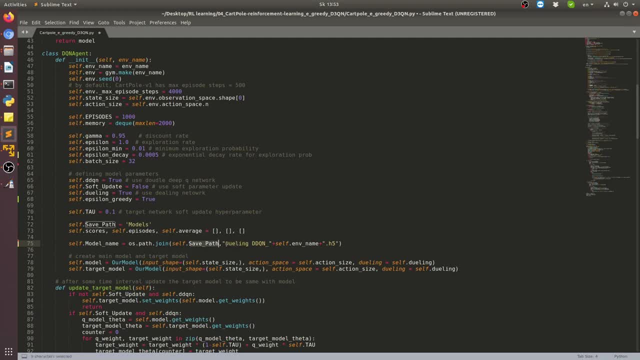 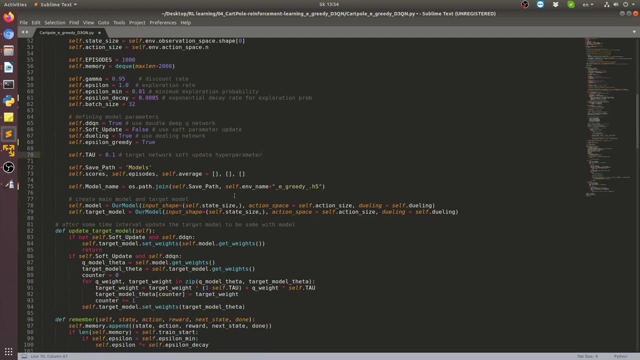 maybe self set path, the same as before, and self environment name. I'll choose this so and right, less what or at the end. but we don't need to set at the end, so I'll use like that and here I'll add a grid, just like that, and yeah at this. 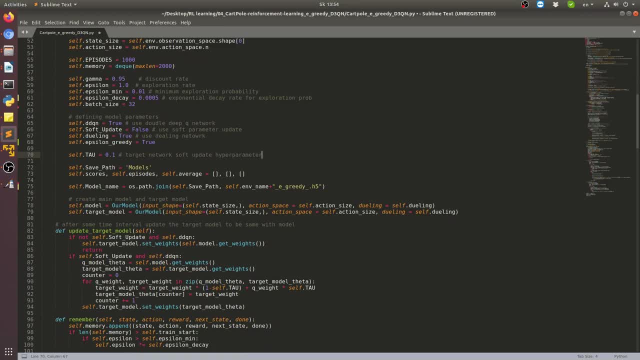 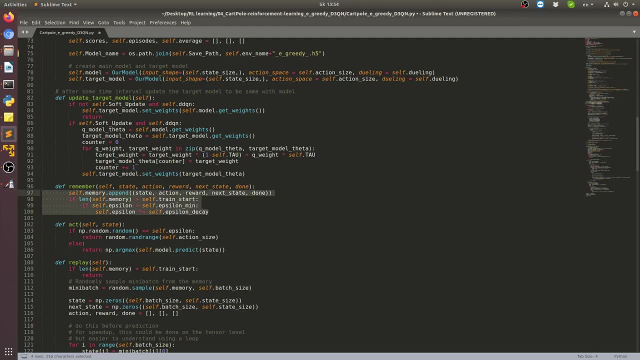 place. that's it. we can move to our remember function. so from our previous tutorial, we had this remember function. right now I'll change this a little bit. so right now it will have some thing like experience and it will be equal to these parameters. experience will be equal. and now what I'll do that I always 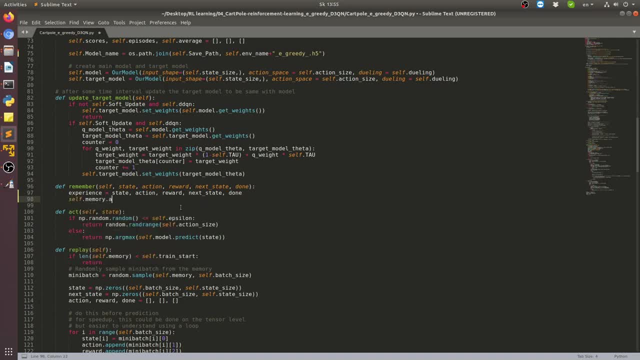 self dot memory dot. append will be experience. experience, just like that. so now what mostly changes is our act function. so before we we are checking if our memory list is equal to self train, start from now on. we'll do our training from our first episode of the game. we won't fill memory with the sample, so we are. 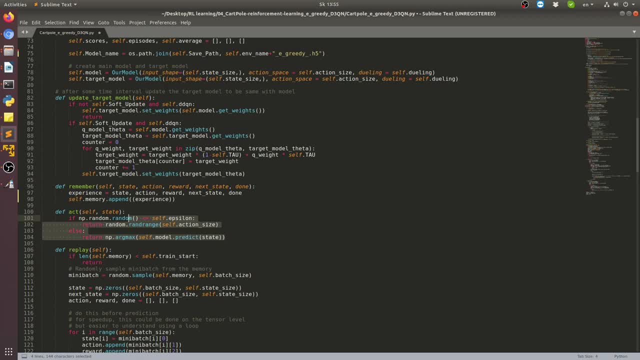 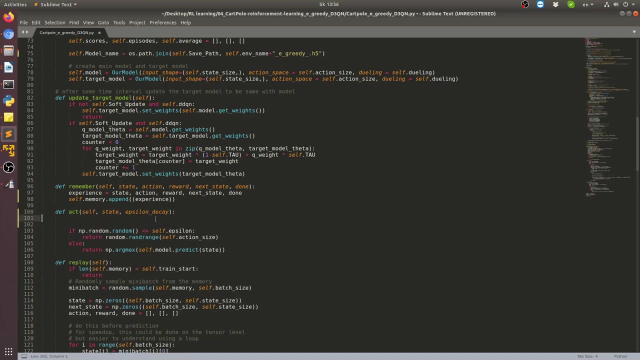 removing all lines and we'll implement absolutely the function in different places. so until now we were having only this. so right now I'll just a little change everything. so now here we'll use our decide step, epsilon decide. before we were not using this, so now, if self dot epsilon greedy, equal to true. so if we choose this, 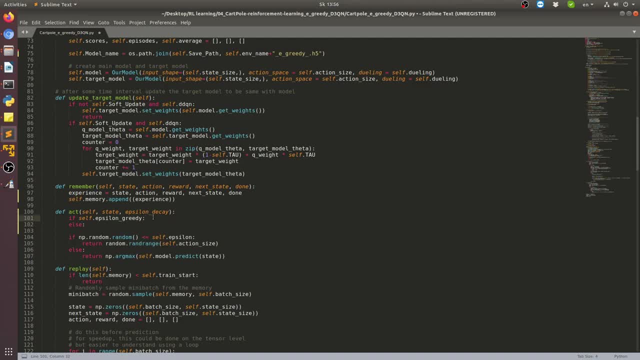 we do this, else we use standard epsilon function as before. so we'll begin from here, so i'll write here: uh, exploration, probability, expo, exploration, exploration or explore, all right, explore me, explore probability for probability, and it will be equal to cell dot: epsilon, epsilon min plus epsilon self, epsilon, self epsilon. 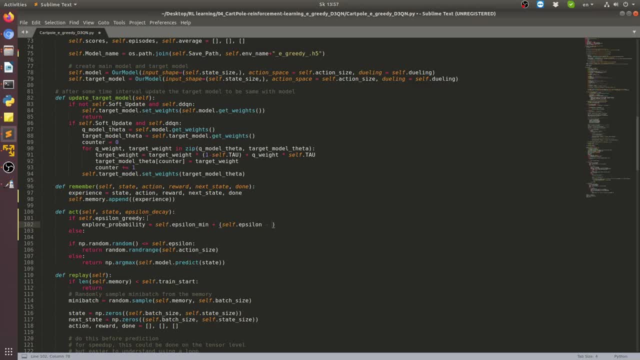 of epsilon, my minus, sorry, minus, epsilon min. epsilon, epsilon min, just like that. and we'll multiply it by numpy exponential and here will be our minus self: epsilon psi. so epsilon psi multiply by psi step psi, where is our epsilon psi step? so uh, yeah, it should be here. epsilon decide, so epsilon psi decide step. 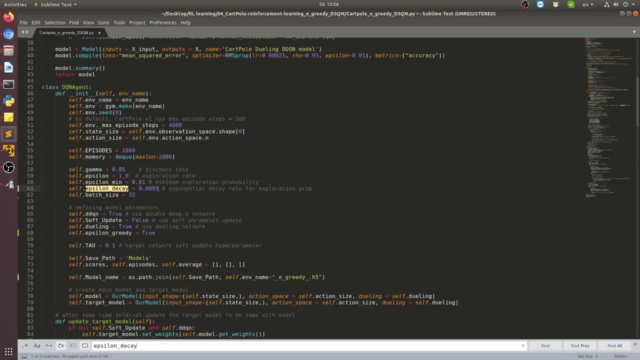 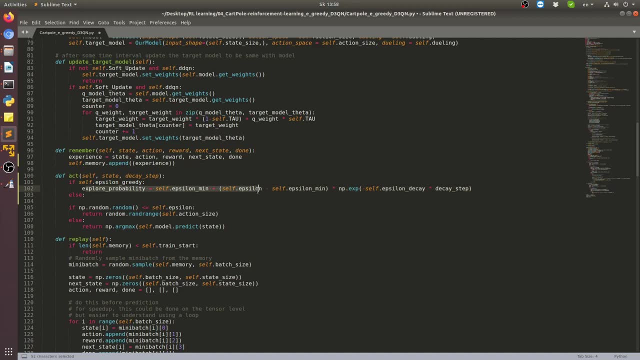 because epsilon decide we have on the top here, yeah, that's right. so now this is only our epsilon grid strategy, and now we would like to return to our previous strategy, for example. so here we just measure: if self epsilon, so epsilon is more than so, epsilon min. 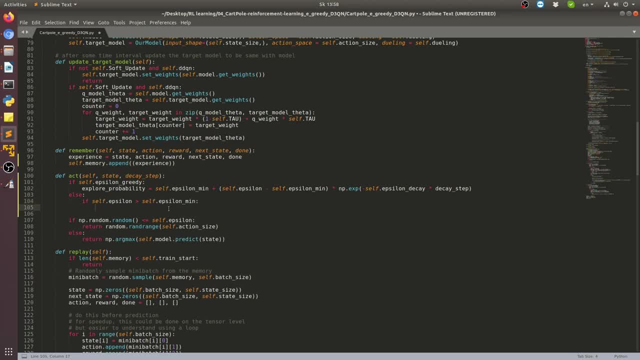 it's like that, one man? and if it is, then we do: uh, self epsilon, so epsilon. epsilon multiplied by one minus of epsilon, the psi, so one minus eps. well, dot epsilon decide just like that, and here our explore probability will be equal to self epsilon. welcome self epsilon. 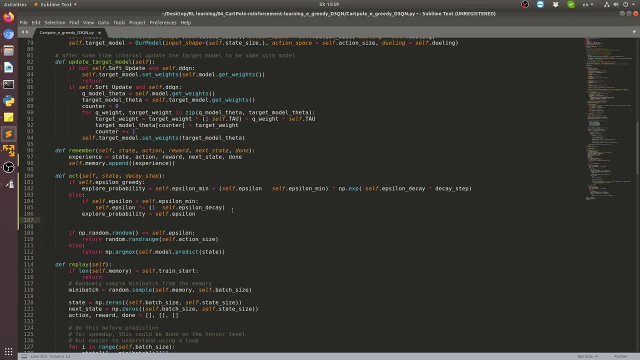 like that. now, if exploration probability is more than random, so something like this, so all. maybe i can choose this. so if explore probability is more than our epsilon? no, i think it's wrong here, so i should have just like that. we'll return a random rand rage as it is here. 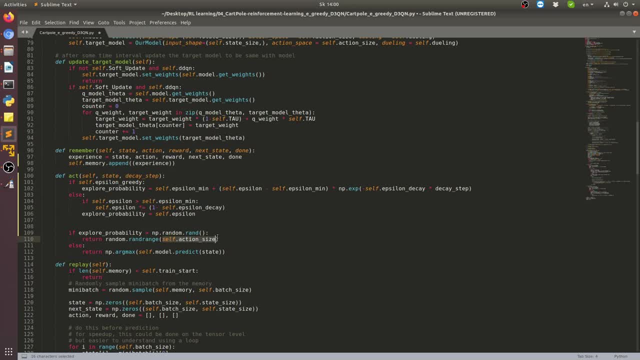 but instead of action site, we actually will add add explore probability, explore probability. so we want to return this and otherwise we also return explore probability here. and, yeah, I think we can minimize this and yeah, we need to add one more tab here. 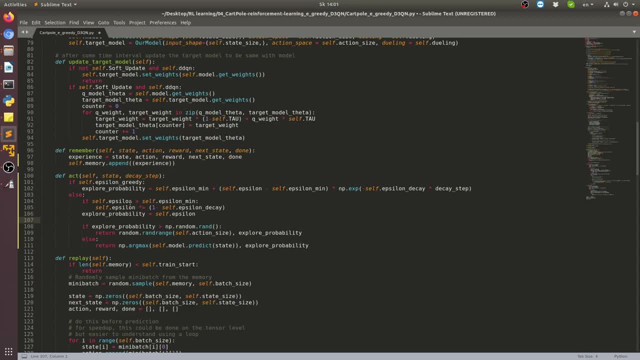 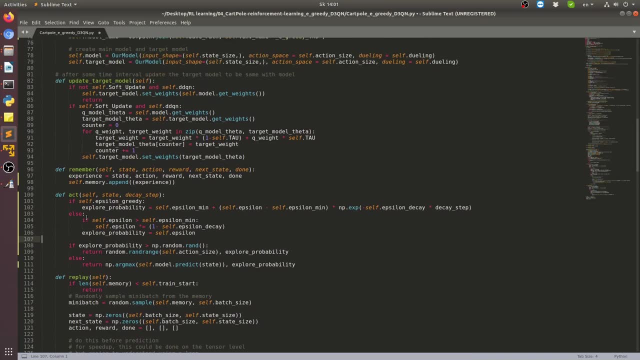 So else or no, I was wrong. we don't need tab here. so that's the idea. and yeah, I think I finished the act function, which changed mostly. so in all code I am removing the self length memory function, so, for example, if I can try find if length self memory train, 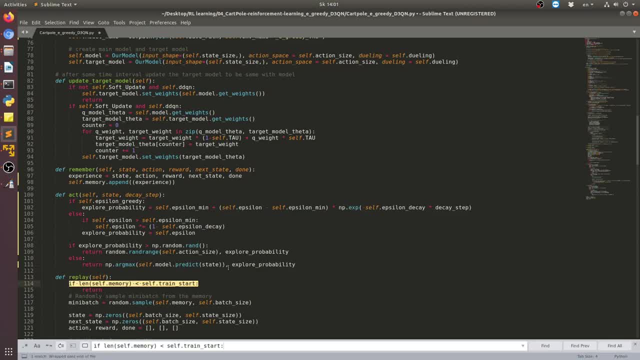 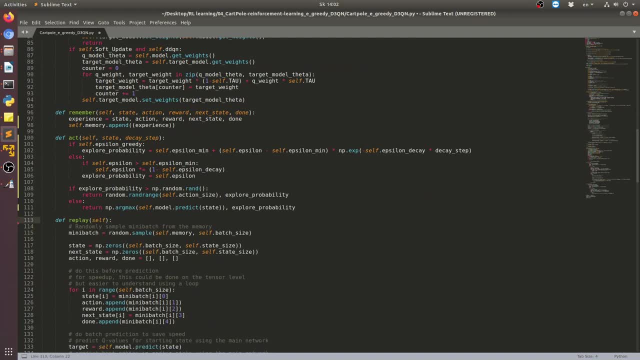 start something like this. I think we don't need to do that. We don't have. we have actually, yeah, we have it only here. so I am removing this in my replay function and, yeah, that's it in what we change in our replay function. 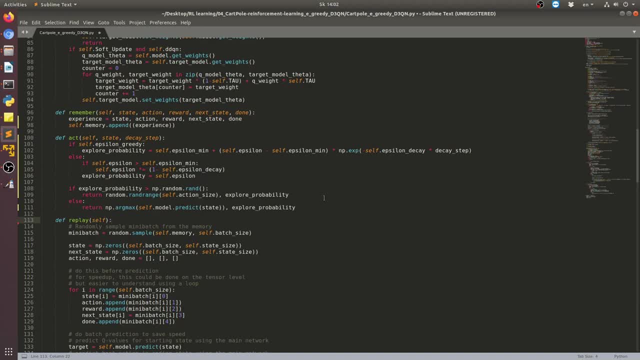 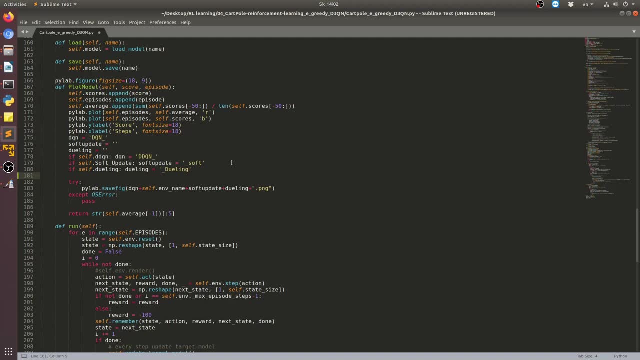 I can. yeah, I almost forgot this. I am adding here additional self epsilon greedy. so yeah, we can do that. so if self epsilon greedy, we write something like that that our greedy is equal to probably greedy, just like that. and here I actually add this as greedy and 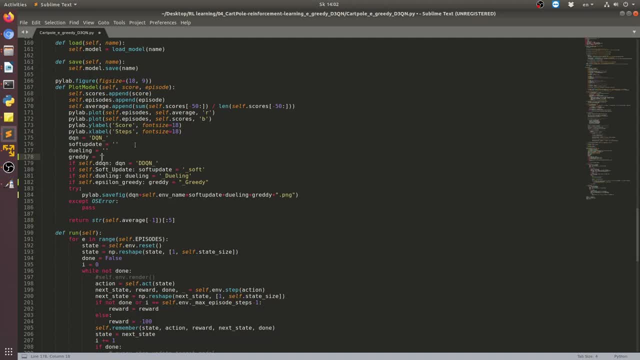 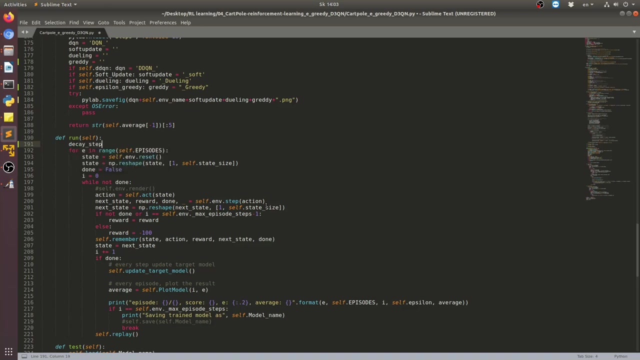 I should not forget to add it here, greedy. so that's it. and now what's left is to change few few steps here in our run function. so here i use a decide decide step x, equal to zero at the beginning, and here i'll add a decide step i, i think. so yeah, side step is equal plus one, and 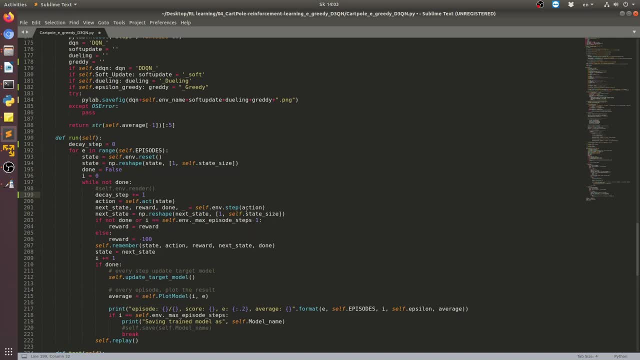 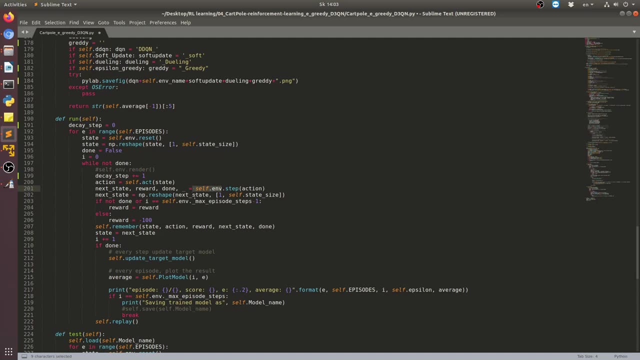 here where i am doing my step and when act. i mean, where's my act here? act, yeah, here is my action and i here add a decide step that i'm sending it to my action function and here i'll add on explore, explore probability actually, and i think that's it what. 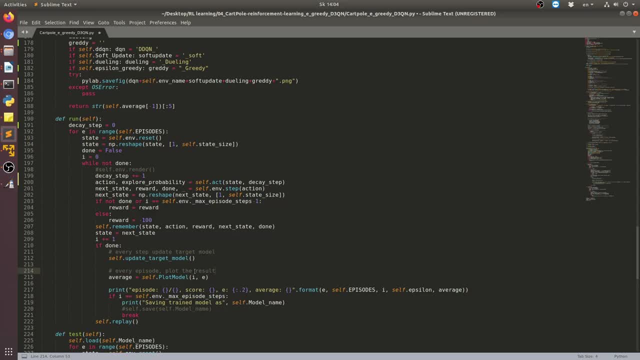 i'm more changing is my print in episodes. so here i have a episode score, epsilon and x average. so right now I'll change this. so I should add explore probability, so instead of i epsilon, so I don't need epsilon here- explore probability, I'll add here. so everything. 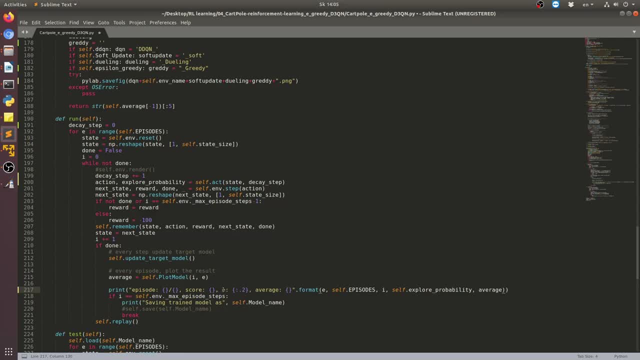 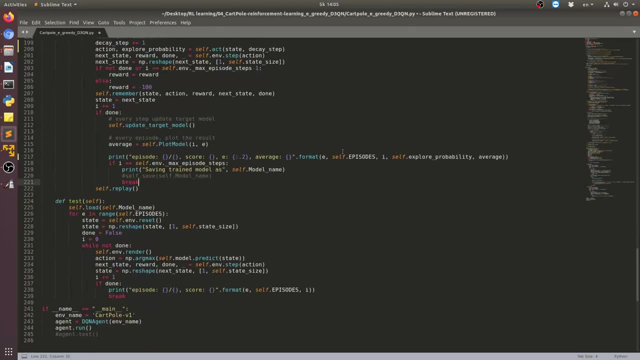 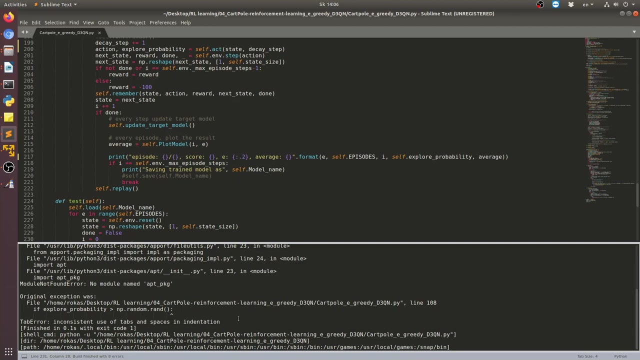 should be quite fine here. but let me think one time. average epsilon: yeah, I think everything is set here. I think I can save it and of course we can try to train our model, probably. ok, I'll just run it and I'll check if we have any errors here. so 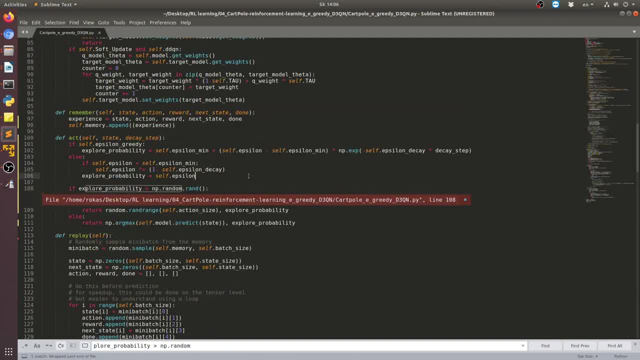 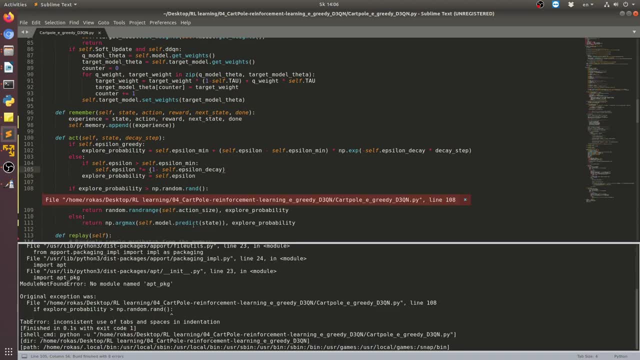 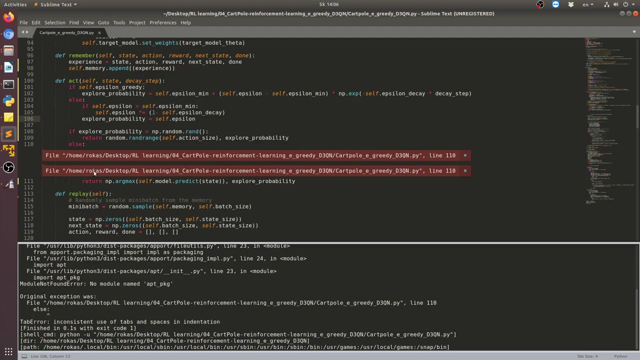 yeah, we have something if explore probability is here. what was the error? I didn't read it. inconsistent use of tabs. ok, yeah, this problem occurs usually on when I use sublime, so I hit this and I don't know usually how to fix this. but yeah, I see that so I've 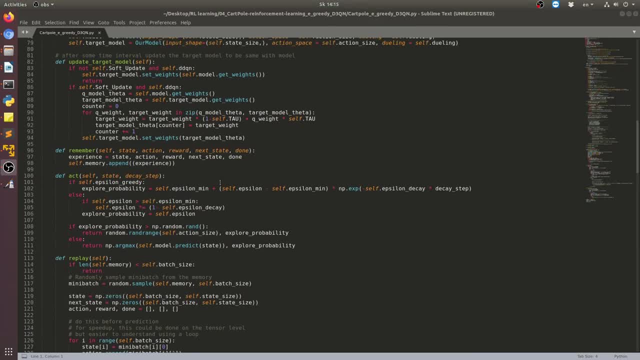 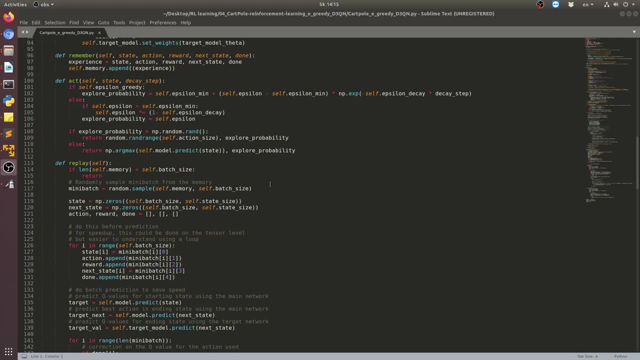 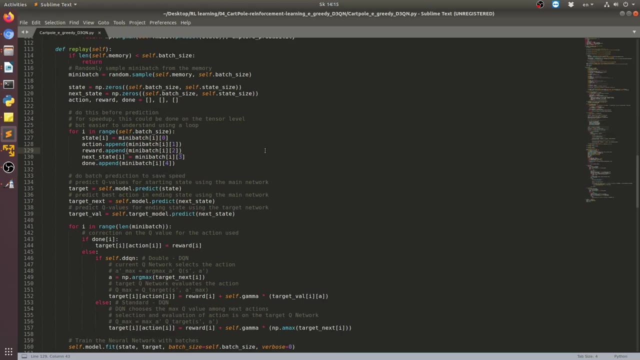 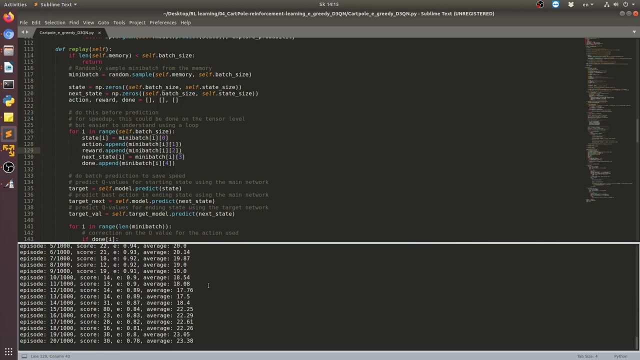 fixed the indentions. Sorry, Sorry for them. and sometimes, yeah, I face these problems, but, yeah, that is the cost of this sublime editor, but in most cases everything is fine. just now I face this so we can actually try to train our model. I build this and that's it.